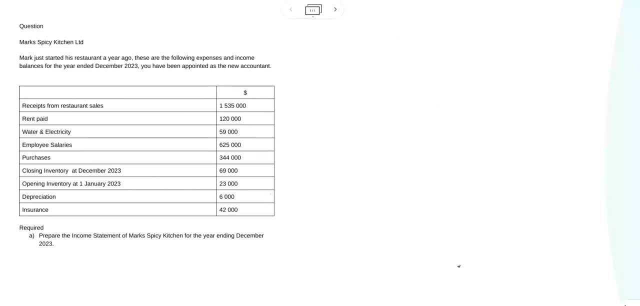 hi. so in this video we are going to do the income statement, but first of all, in this video we're just going to focus on the cost of goods sold and how to calculate it. so the cost of goods sold is what you actually need to calculate your gross profit and, in turn, your net income. so first of all, when you do your 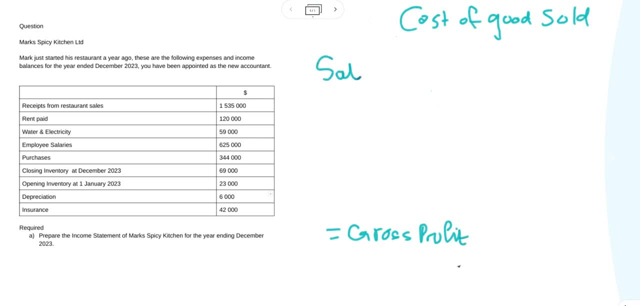 income statement. you always start off with your sales. so in this case our sales are 1 million 535 thousand. and now we need to. in order to get to our gross profit. we need to calculate what our cost of goods sold is, so we will have your sales less your cost of goods sold, and to get the cost of goods also when 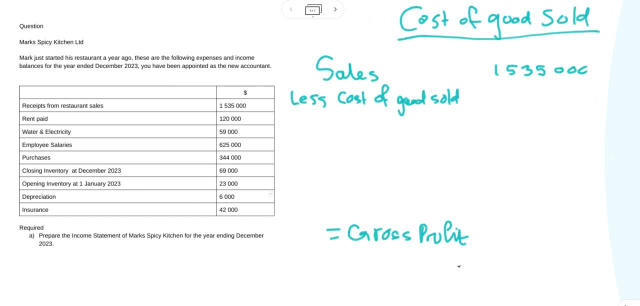 you're selling an item, you sell it at a certain price, so for the cost of goods. so we just want to find out how much did it actually cost for us to make the sales or to make the, the products that we are selling off? so less your cost of goods sold is your. 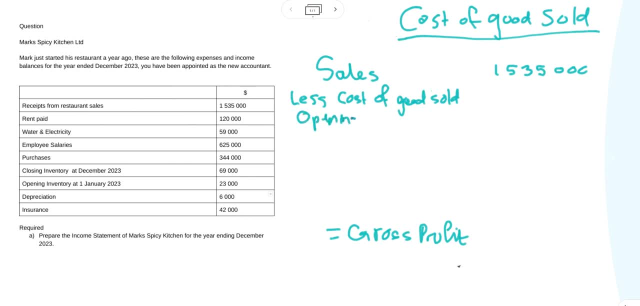 opening inventory or your opening stock, meaning the stock that you have at the beginning of the year that have not been sold yet. so in this case our opening inventory is 23,000, so we have your 23,000. then we are going to add your purchases because 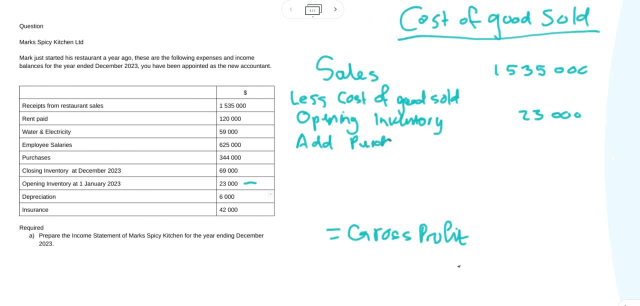 now we're buying more things, so we need to add the cost of the- the goods that we bought during the year, and in this case, our purchases is three hundred and forty four thousand, and then we need to deduct that. we need to deduct your closing inventory because this was already accounted for in the previous year. okay, 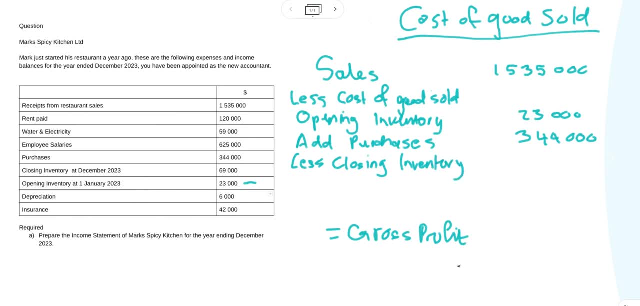 because in the previous year we also had your- what do you call it? where we also had that. so now your closing inventory will be your 69,000. now if we get all of this, we are going to find your cost of goods sold. so we have your.